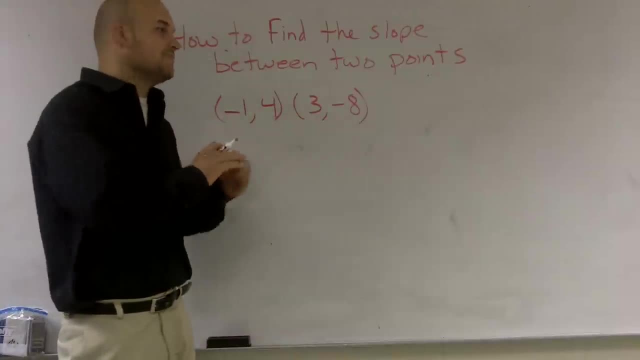 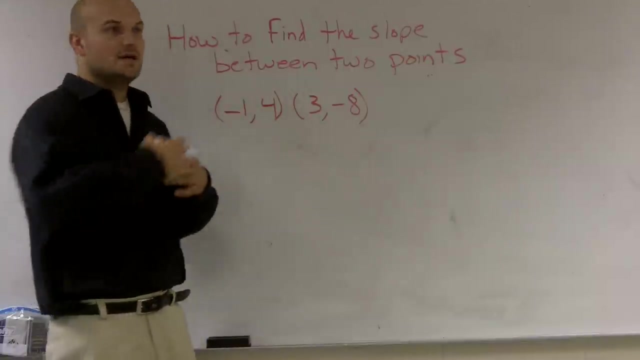 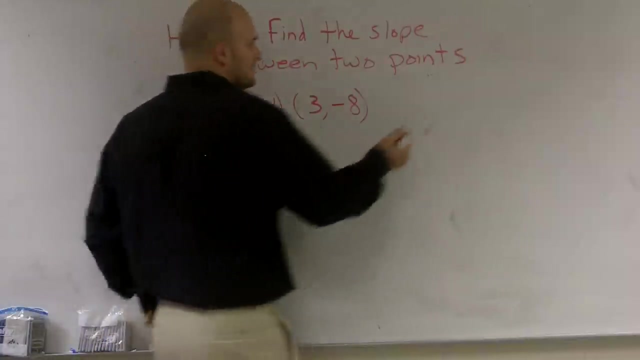 over run is how much between two points, how far? what is the distance that your graph or your change in elevation is risen and how far has it gone left or right? So we need to go ahead and define that distance, We need to find the change. So let's go and 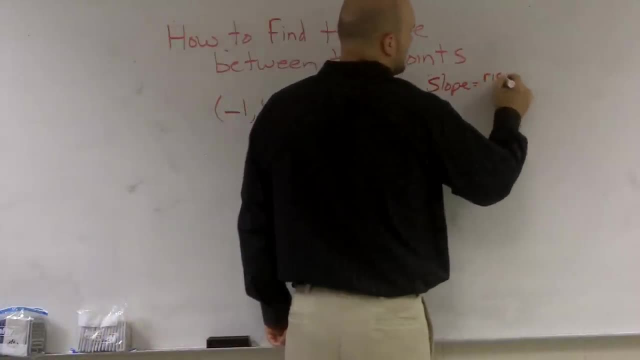 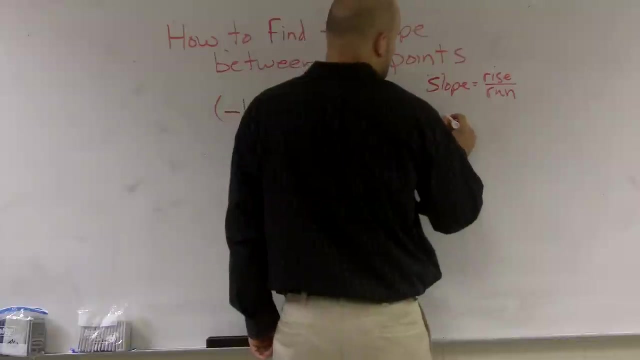 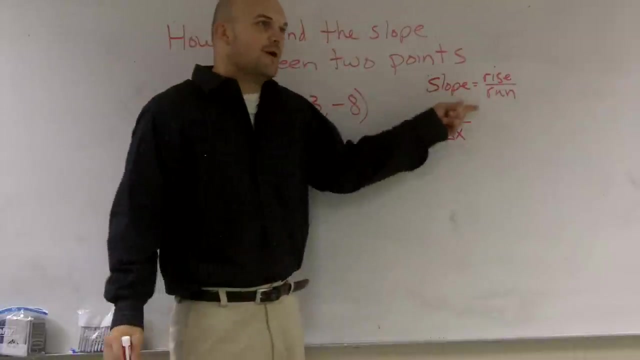 look Slope, very commonly referred to as rise over run, And what does that really mean? What is really the rise or run? Well, what that really is is the change. we're going to write as delta y over delta x, And what this means is the change in y over the change. 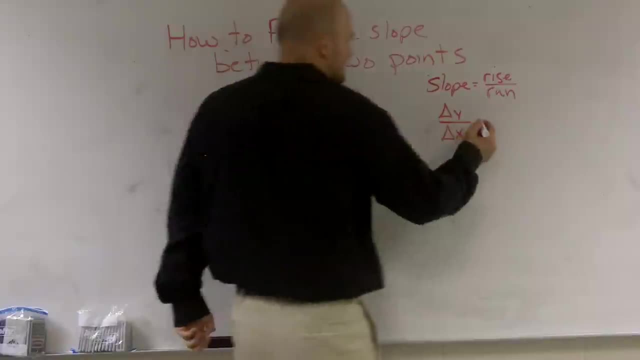 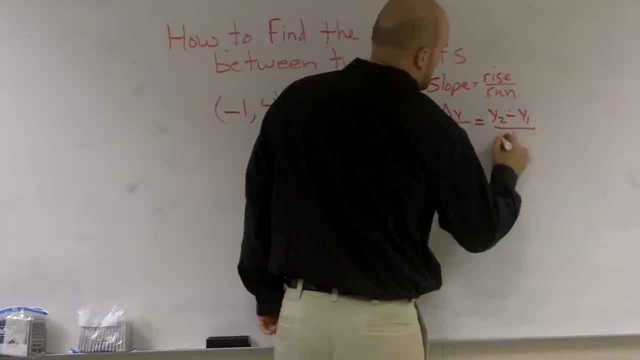 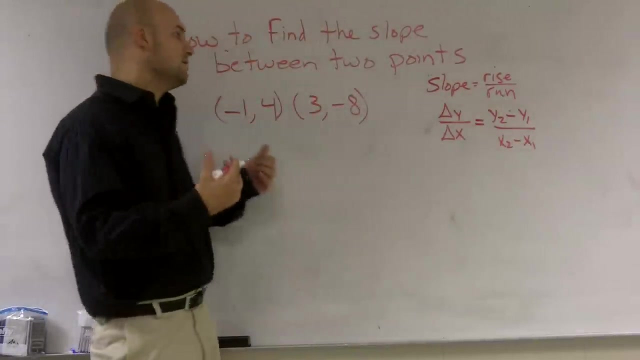 in x. Well, that's kind of craziness. Give me a better thing, Give me a better way to write this, All right? Well, if we have two points, we can label our points x1, y1, and x2, y2.. So 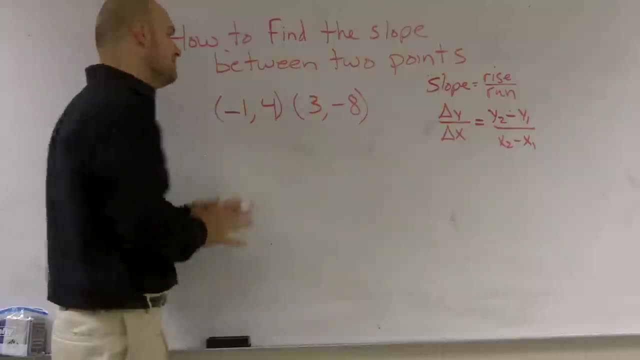 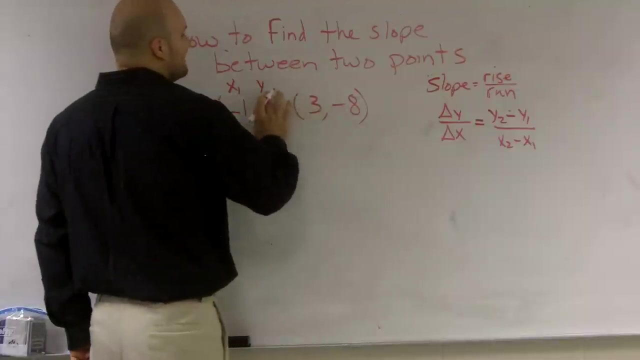 I'm going to look at these two points and I'm going to go ahead and label them. It doesn't matter how you want to label them, which one's x1 and which one's x2.. But I'm going to say this one would be x1 and this one's y2.. Well, I won. This one is x2 and this one is y2.. 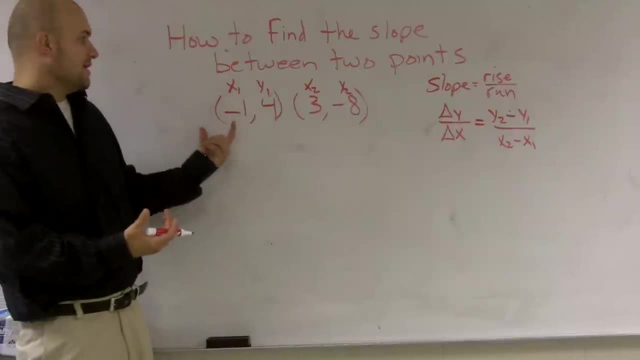 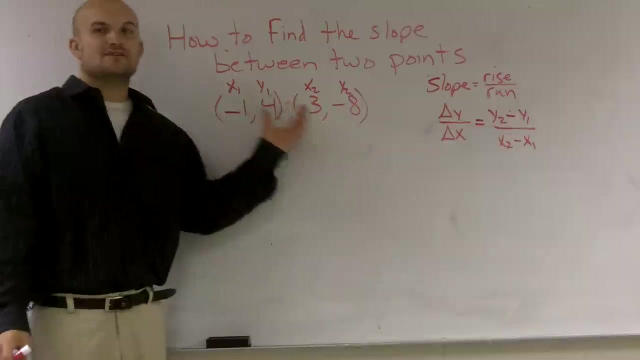 Okay. So because you remember, on a coordinate point you have your x and your y, Your x and your y. However, you can't both label these x and y, so we use subscripts to differentiate between the two points. All right, So now, if I know that my slope is the change in y, 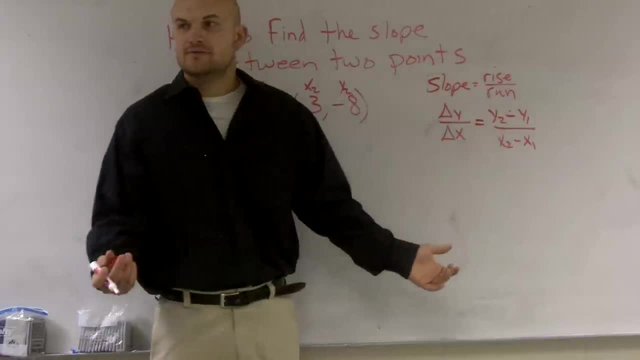 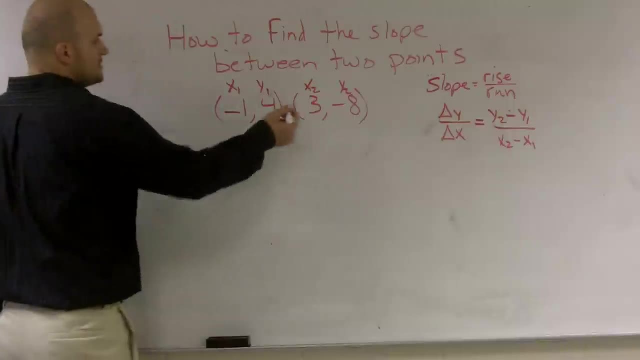 over the change in x. all I'm going to do now is just like we learned before. Now we're just going to evaluate and plug in our values into our equation for slope. All right, So I just take my y2, which is a negative 8.. 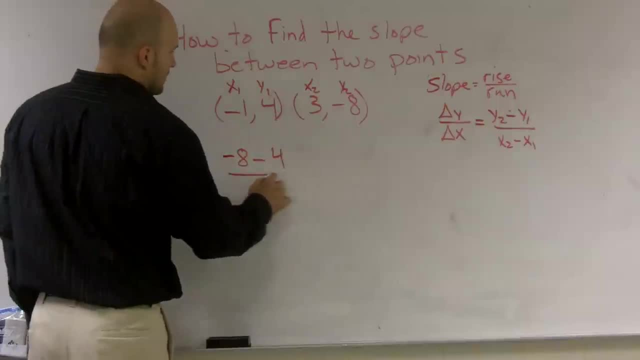 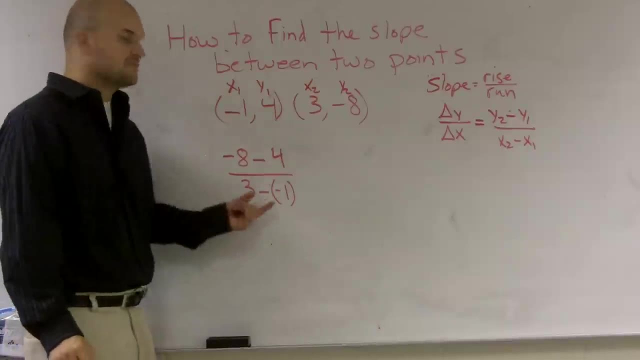 Minus y1,, which is 4.. All over x2, which is 3. Minus, I'm going to put in parenthesis a negative 1.. Remember, I'm going to keep those parenthesis just to make sure that I'm. 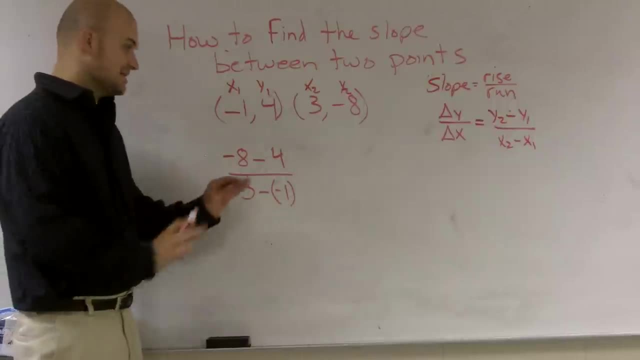 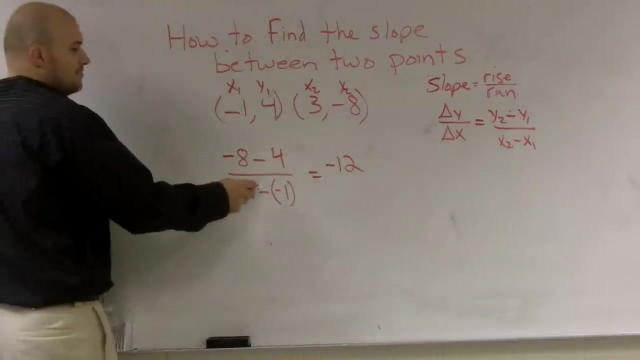 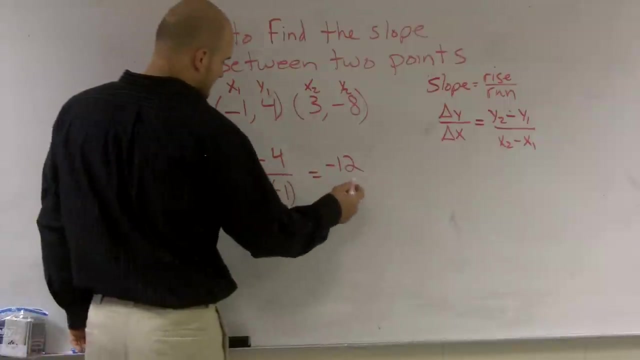 not making any mistakes, Making any mistakes with my negatives. So a negative 8 minus 4 is going to become a negative 12. And 3 minus a negative 1. These are going to the two negatives are going to cancel each other out and it's going to become a positive negative.